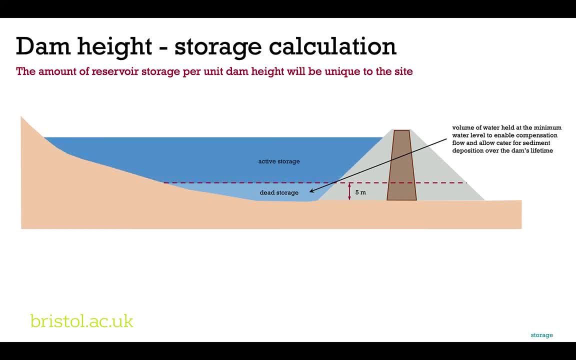 Then, above that minimum water level, is what we call the active storage, and this is the storage volume that you have calculated To meet the demand With a 1% probability of it failing in any given year. So that is the value you've calculated. there is the active storage. 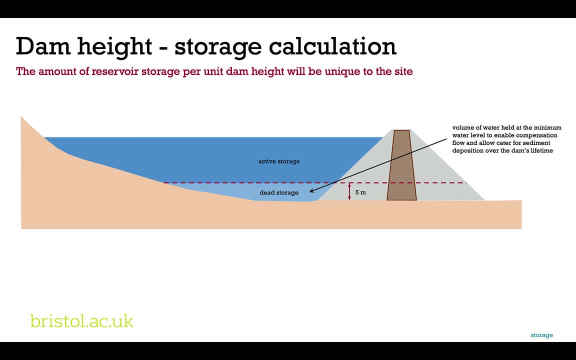 And so, in order to figure out what height of dam you need, you're going to have to consider both the dead storage and the active storage. Now just a quick note about two other parts of this water balance. First of all, you would expect to lose water from evaporation from the surface. 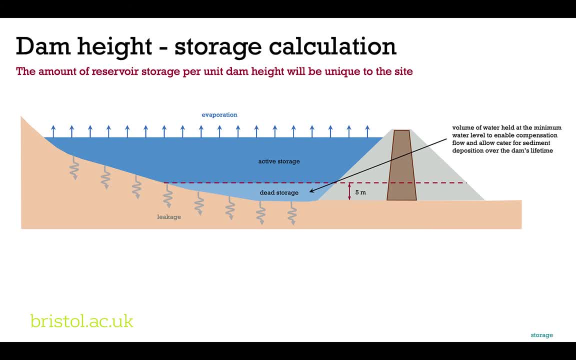 Of the reservoir and you might expect to lose some from leakage From the, from the base, And because of the particular circumstances of the valley and the additional levels of complexity that will be required for your calculations, We are saying that you don't have to consider evaporation and you don't have to consider leakage. 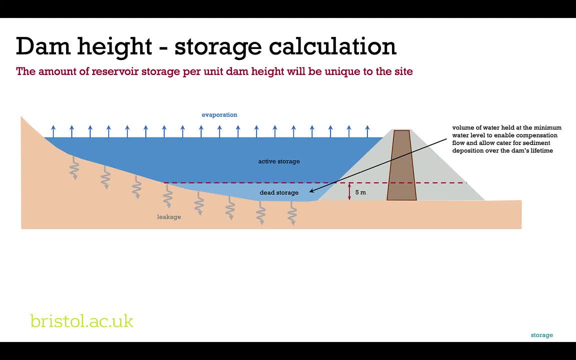 These will be minimal compared with the broader volumes that you're going to be thinking about, And so you don't have to consider those as part of the feasibility study. Okay, so how do you go about determining the height of the dam in order to provide your active storage and this dead storage? 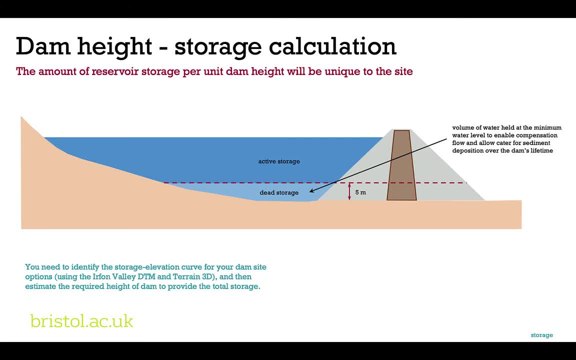 Well, what you need to do is to identify something called the storage elevation curve for your individual dam site options, And you do this using the Irfan Valley Digital Terrain Model, the DTM and Terrain3D. I've provided these for you on Blackboard. 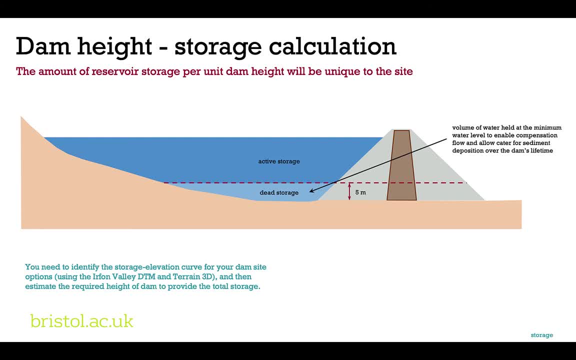 The Terrain3D is an executable program for Windows And you feed into it the Irfan Valley Digital Terrain Model DTM as an input And then you have to specify where you want to put your dam And it will draw your storage elevation curve for the landscape behind your specified dam site. 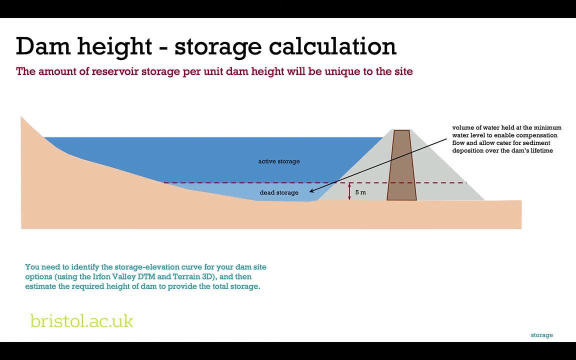 So once you've done this, you then need to figure out what height of dam you need in order to produce the active storage And also to produce the additional storage in the dead zone from the design specification given here.